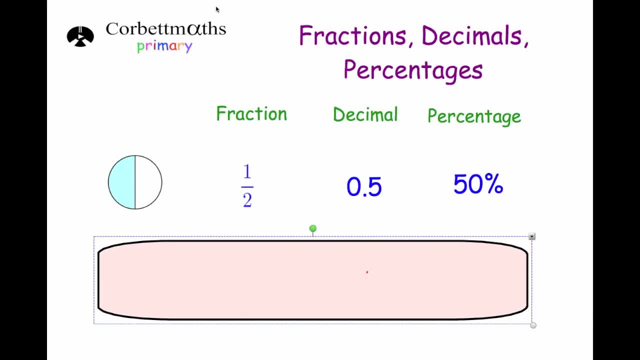 OK, next. so we've done one half, now let's have a look at two halves. So, as you can see, this diagram represents two halves, because both of the halves are shaded in. so as a fraction, that would be 2 over 2.. As a decimal number, that obviously that's a whole, because all 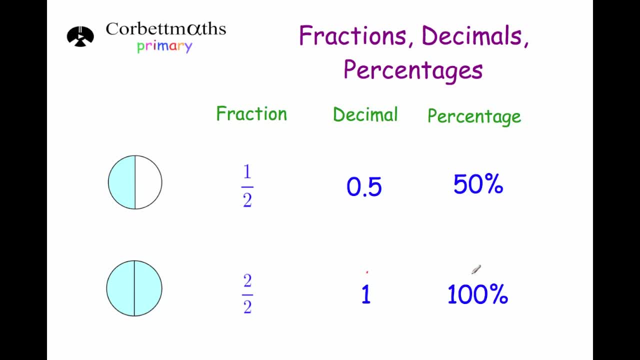 of it is shaded in, so that's 1 and as a percentage that's 100%. Any time a fraction has got the same number on the top as the bottom, that is one whole, because obviously three thirds or 4 thirds are golden quarters, or five fifths would all be a whole. okay next. so now we're going to. 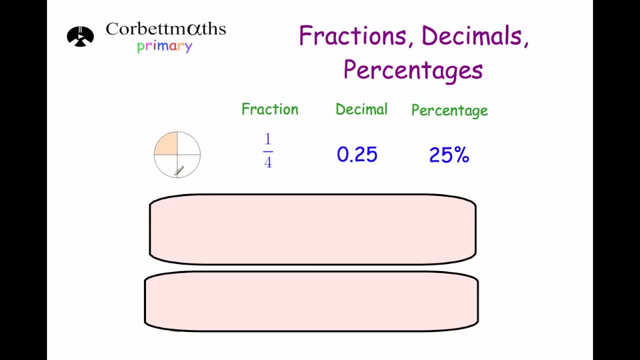 move on to quarters. so first of all, one quarter. this diagram represents one quarter because one of the four sections is shaded in, so that's one over four. as a decimal number, that is not 0.25, and as a percentage, that is 25%. okay, so that's. 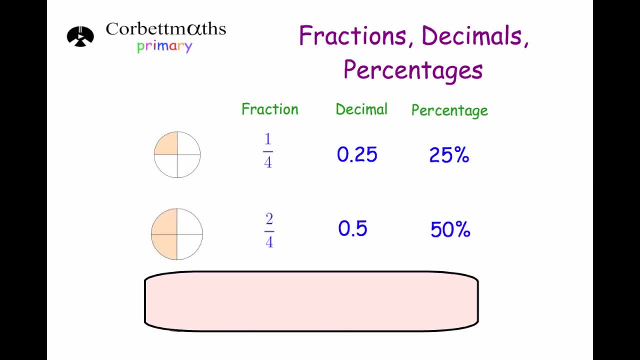 one quarter. okay, that's a very important one to learn. our next one? our next one is two quarters. now, two quarters. as you can see, we've shaded in two of the four sections. that's the same as a half. so as a decimal number it's not 0.5, and as a 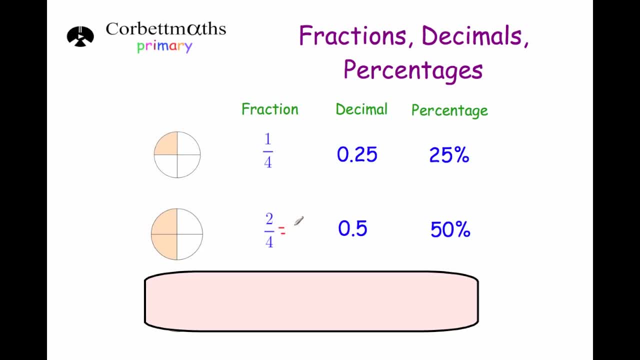 percentage is 50% and two quarters is the same as a half, because obviously it's an equivalent fraction. it could be cancelled down, so that means it's two quarters. you probably wouldn't see that as often because it probably be just written as one half, which is not 0.5 and 50%. okay, next, another very important one. 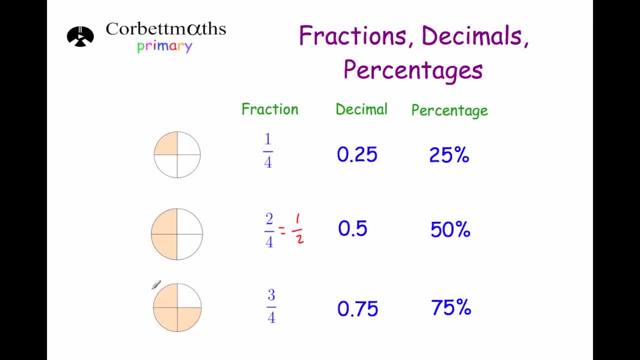 is this one which is three quarters. this diagram represents one quarter and this one is two quarters, and this one is two quarters. three quarters because three of the four sections are shaded in, and three quarters is not 0.75 and, as a percentage, 75% because, obviously, if half of it is, 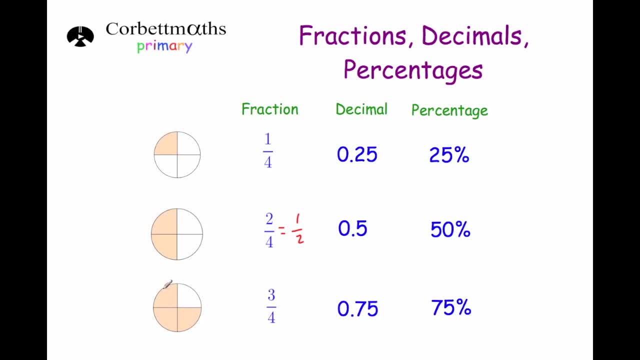 50% and the other one is 25%. all together, that would be 75%. okay, so these two, the one quarter and the three quarters, these are very important facts that are like the half as well. the half is extremely important. okay, next let's. 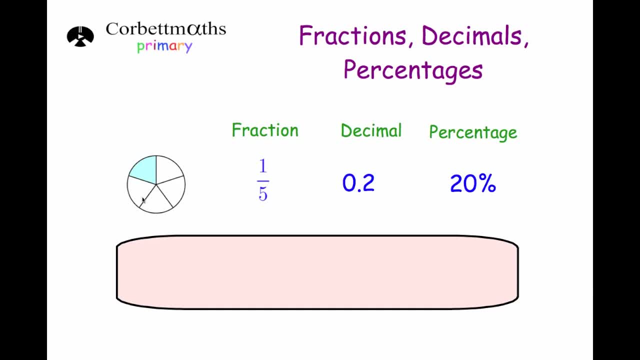 have a look at fifths. so here we've got a circle, we've got five sections and one of them is shaded in, so that represents 1- 5th. as a decimal number, 1 divided by 5 is not 0.2, and as a percentage, obviously, 100% divided by 5 is 20%. so each of. 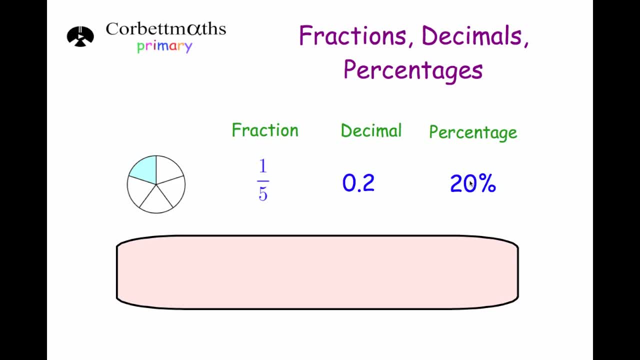 these sections is 20%, so one of them would be 20%. okay, so that's one fifth. again, that's another important one, that's important to learn. next, one, two fifths. well, if each section is worth 20%, two of them would be 40%, so this is two. 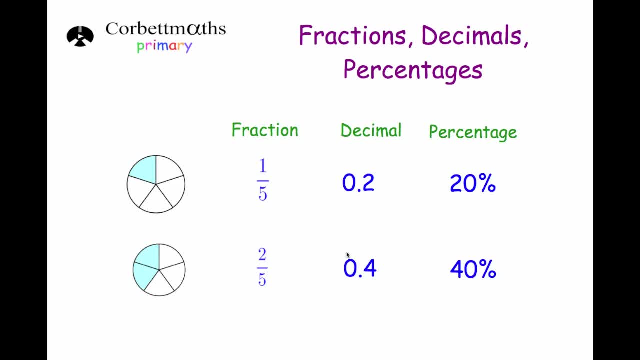 fifths, and that's the same as 40% as a percentage and as a decimal number. that would be, if each one of them is not 0.2, that would be not 0.4. so each section is not 0.2, so two of them is not 0.4. again, that's another important one I would. 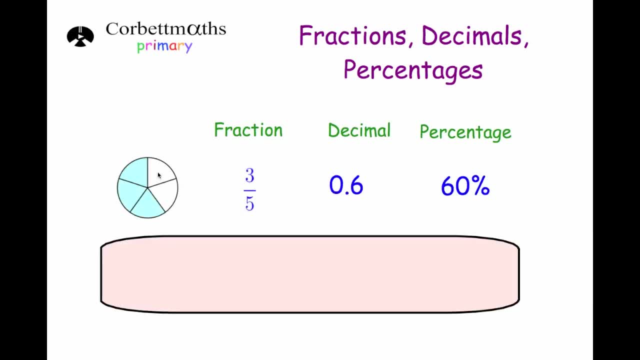 learn all the fifths. they're quite important. our next one, three fifths- well, that's gonna be not 0.2, not 0.4, and not 0.6 as a decimal number, not 0.6, and as a percentage, that would be 60%. and our last fifth, though, is very important. 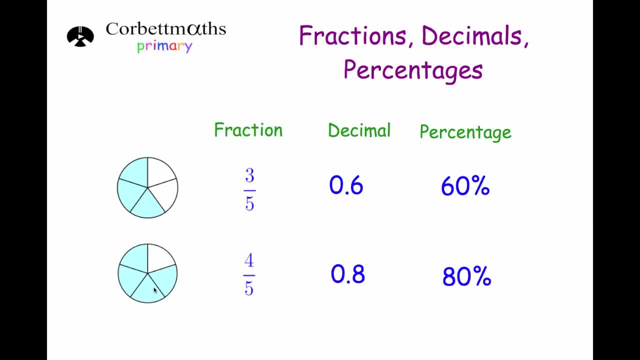 because obviously five fifths, as a whole, four fifths would be not 0.8, because not six, not 0.8, and that would be 80%. so each fifth is 20%. so if you remember that, you should be able to remember all the fifths. okay, so we've gone through halves. 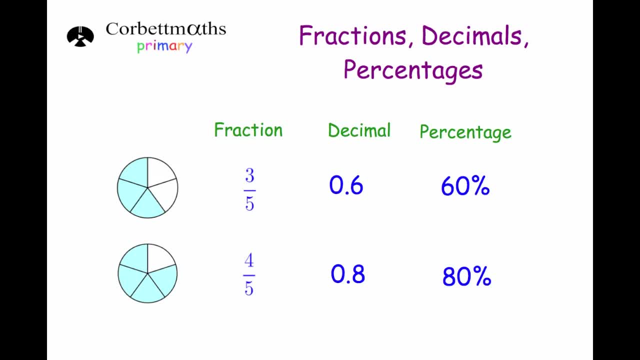 we've gone through quarters, we've gone through fifths, now we're going to go on to tenths. now here we've got one tenth. we've got ten sections, and one of them is shaded in, so that represents one tenth. one divided by ten is not 0.1, and 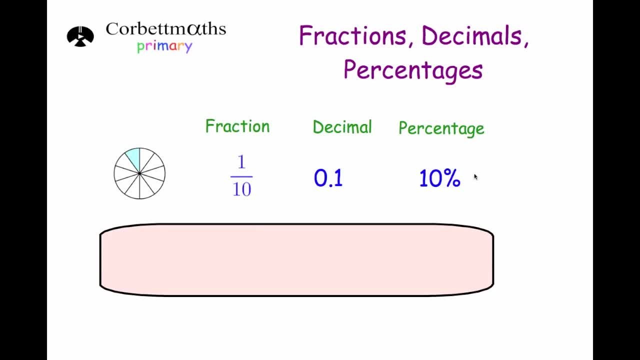 as a percentage. well, a hundred percent divided by ten is ten percent. so each of these sections is going to be ten percent or not 0.1. so we can use that to work out all of them. so our next one, our next one, is two tenths. now, two tenths of each section is ten percent, ten percent, twenty. 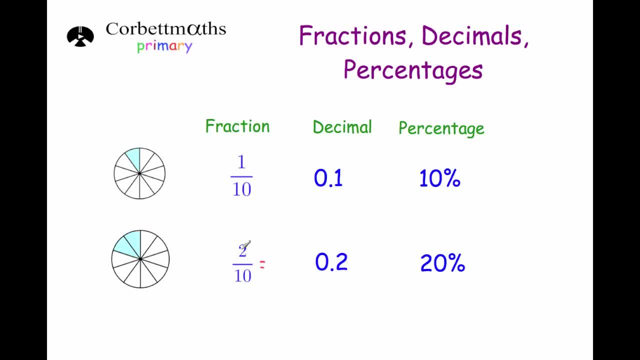 percent. now we've already had that already, because two tenths, if we divide both of those by two, would be one fifth. so two tenths is just one fifth. so we've seen this one already. okay, so one fifth is not 0.2 and twenty percent, and that's. 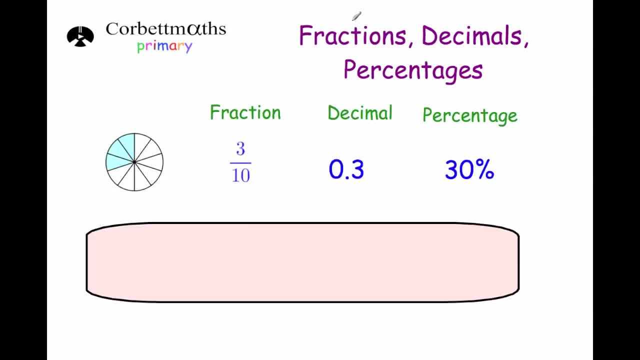 the same as two tenths. okay. next three tenths, well, that would be another ten. so as a percentage, thirty percent and as a decimal number, 0.1, 0.2, 0.3. so three tenths is 0.3 and thirty percent. four tenths, well, that would be 0.4 and forty. 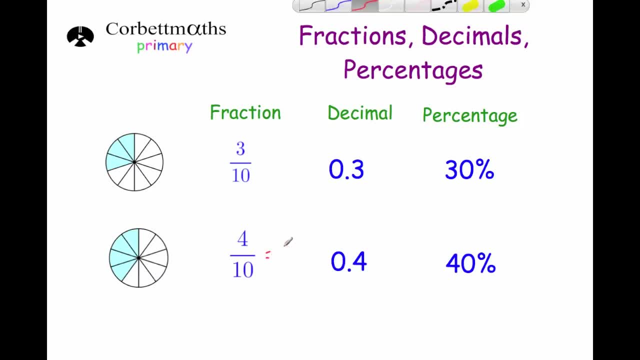 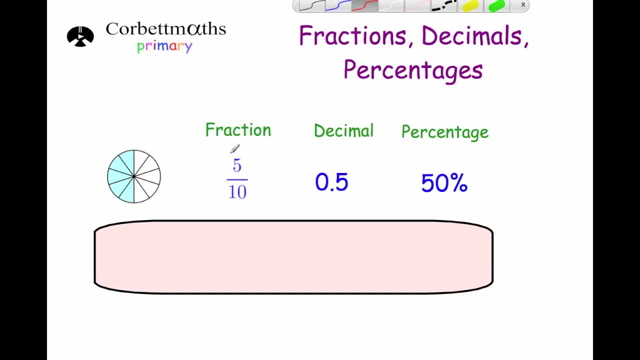 percent, but that does cancel down. we have had this one already. that would be two fifths, okay, so two fifths is also no point. four and forty percent, our next one, five times. as you can see already, that's the same as one half, which is no. 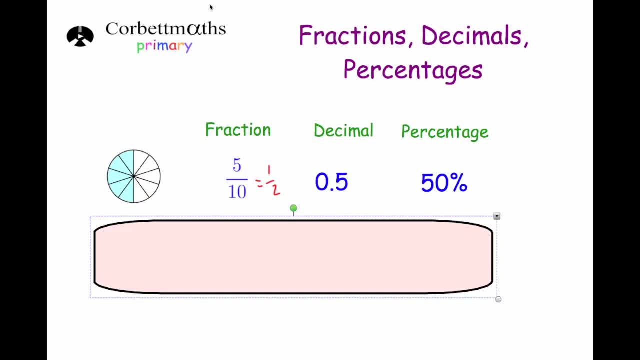 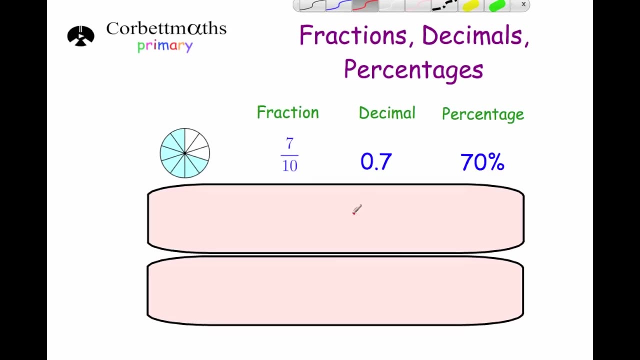 point five and fifty percent and six tenths. if we ever look at it is also no point. six and sixty percent, that's the same as three fifths. our next tenth is seven tenths. well, seven tenths would be no point. seven and seventy percent, our next one would be eight tenths, which? 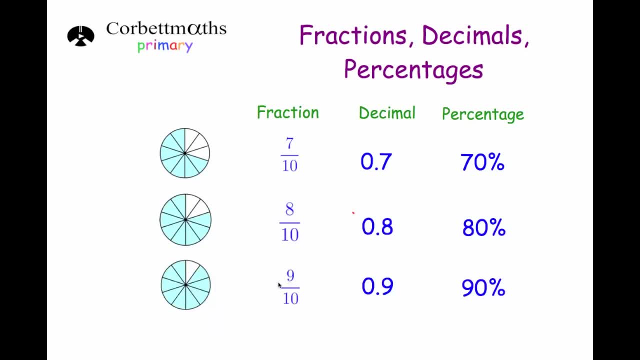 is going to be no point. eight and eighty percent and nine tenths, which is no point. nine and ninety percent. so there the temps. temps are quite nice actually, because the number on the top of the fraction will just become the percentage. you know, you just turn like we're just times by ten, so like seven. 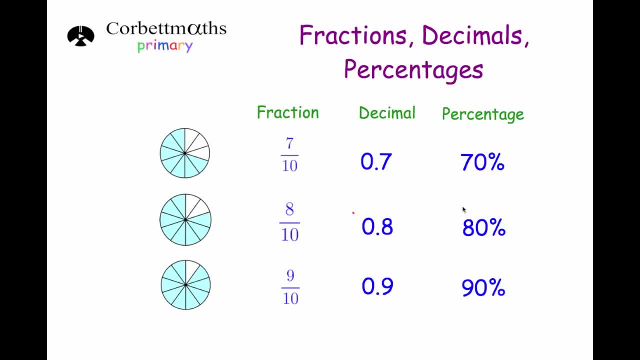 over ten is the same as seventy percent, eight over ten is eighty percent, nine over ten, ninety percent, and as a decimal number it'll just be no point on whatever whole numbers above the ten. okay, and finally, we've looked at halves, we've looked at quarters, we've looked at fifths and we've looked at temps. we're. 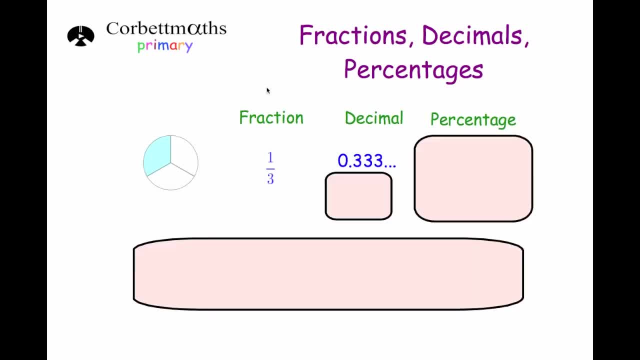 now going to look at thirds. now, thirds are quite an interesting one, because we can see this diagram. it represents one third. one of the three sections is shaded in, so it's one third. and then we've looked at thirds and we've looked at quarters. now, if you do one divided by three and if you use the bushelter, 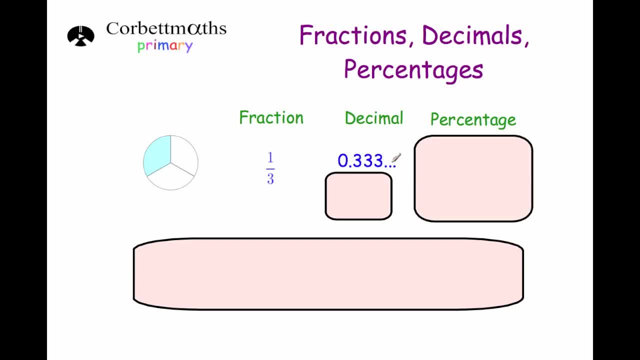 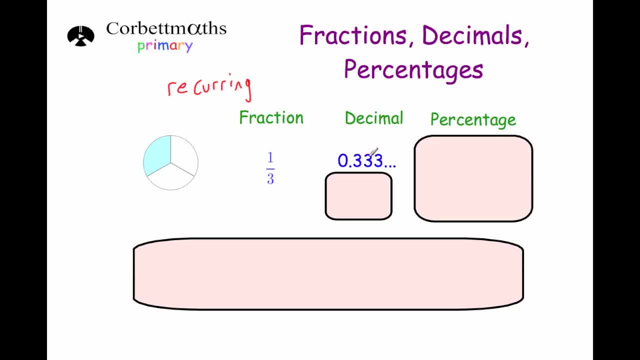 forever. but I would just write no point three, three, three and three dots, just to show that it carries on. there is another way to do that. it is to write 0.3 and a little dot above it. that's the recurring symbol, and if you put it, 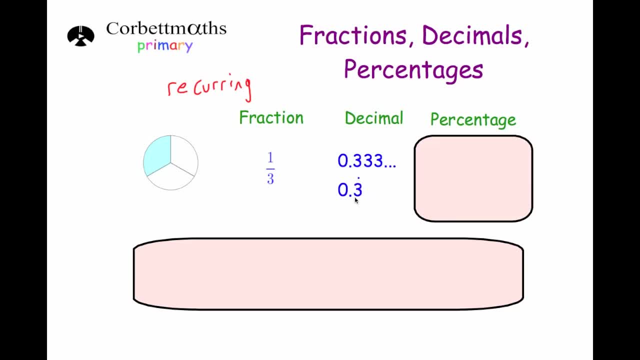 above the number that repeats forever. it just means the person looking at it will know this means 0.3333 and so on. it's very important that you do spot it though, okay, because it's not the same as 0.3, it's 0.3333 and so on. now the decimal number goes on forever, so that means the percentage.